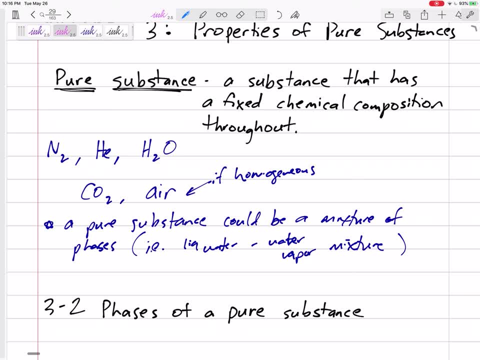 So a pure substance could be a mixture of phases, as long as, As long as Everything in the mixture, As long as everything in the mixture Vaporizes at the same temperature, For example air. If air, for somehow, was changing from the phases, all the different. 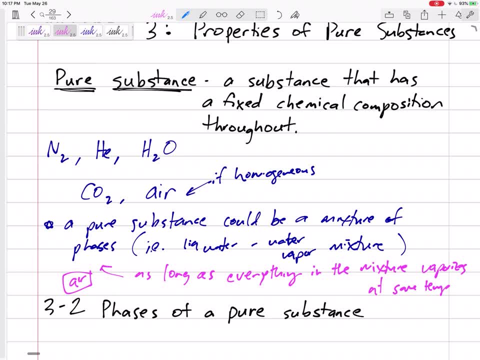 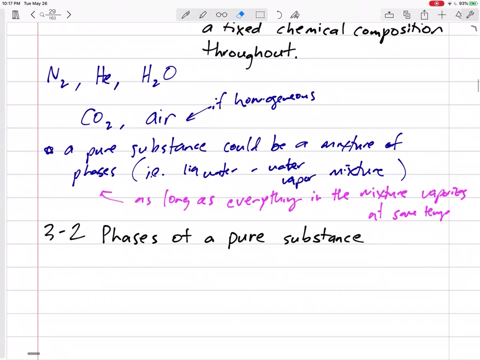 All the different chemicals in the air might vaporize at different temperatures, and so if one vaporized before the other, then it's no longer a constant, fixed composition throughout. so but one thing that is is water, water and refrigerant, those we can have mixture of water and vapor, and it is still a pure 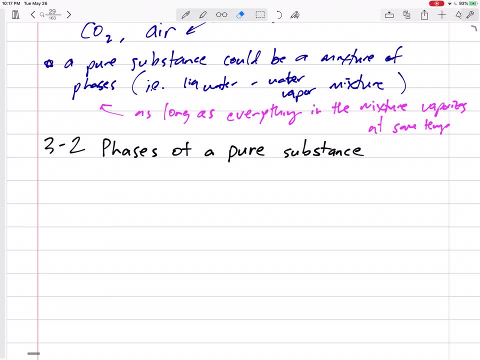 substance. okay, obviously the phases of a pure substance would be solid, liquid and gas. you know that. but but we, we want to make a note that for solids and liquids there's not much change in volume with heat compared to a gas. you know that, but but we, we want to make a note that for solids and liquids there's not much change. 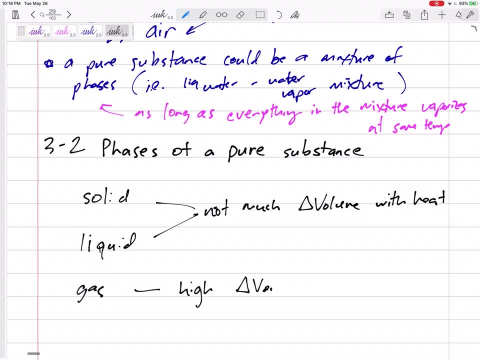 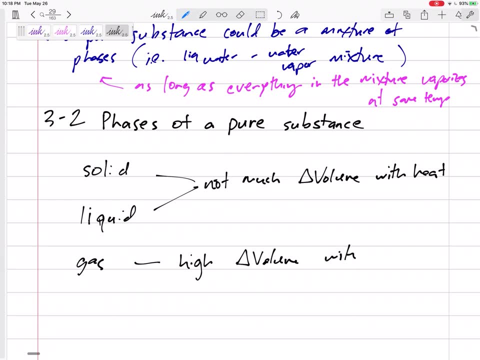 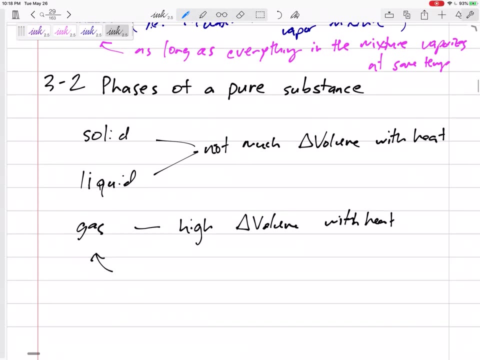 in volume with heat compared to a gas. you know that. but but we we want to make a note that for gas very high change in volume, very large change in volume with heat. okay, we'll talk about this later, but for gases, gases are kind of very different than liquids and solids obviously. 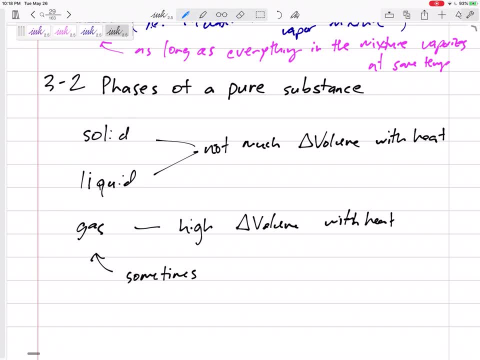 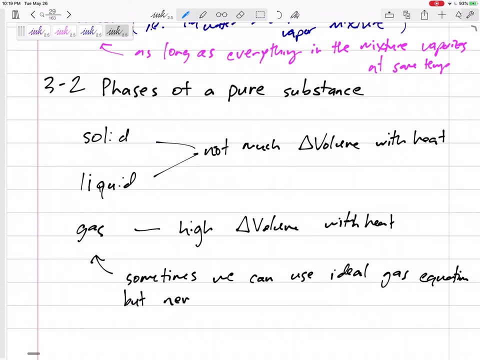 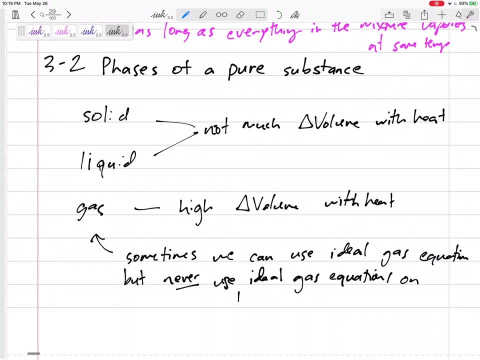 we can treat them differently, and sometimes we can use the ideal gas equations. sometimes we can use the ideal gas equations, but never use those idle gas equations for liquid gas equations or solids. right, i mean, that seems obvious, but sometimes we're just not thinking. if it is a liquid, don't use ideal gas equations or never use idle gas equations. on.